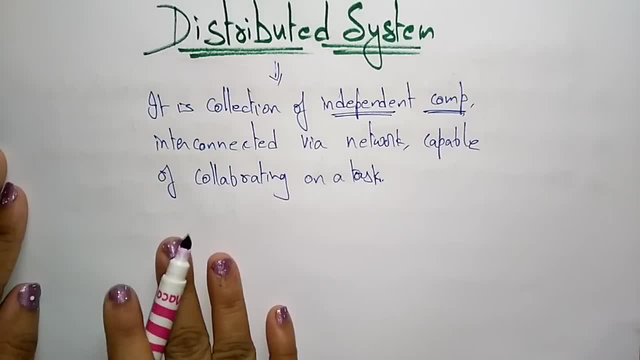 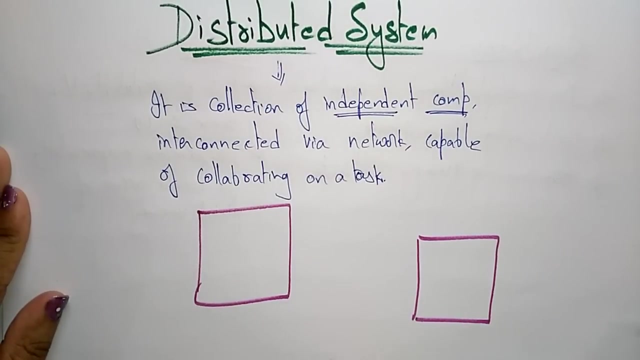 It means one system is depends upon another system, So that is a tightly coupled, Whereas the distributed system- here we are taking a collection of independent computers interconnected via network, and those systems, those computers, are capable of collaborating on a single task. So here let us take: this is one and this is one and this is one. Suppose we are taking a different, a different system. 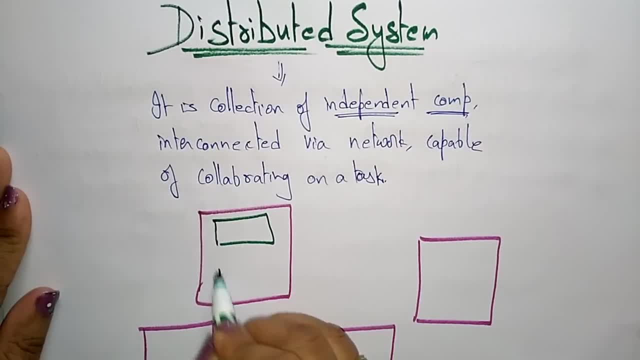 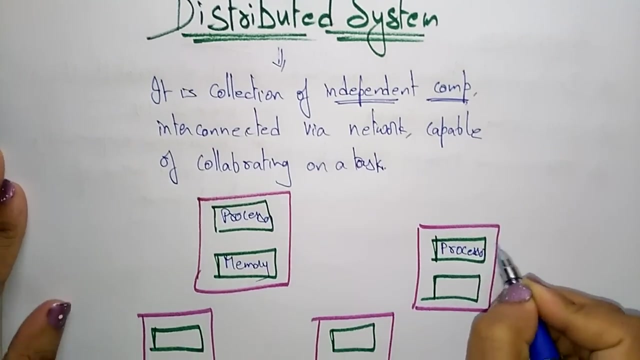 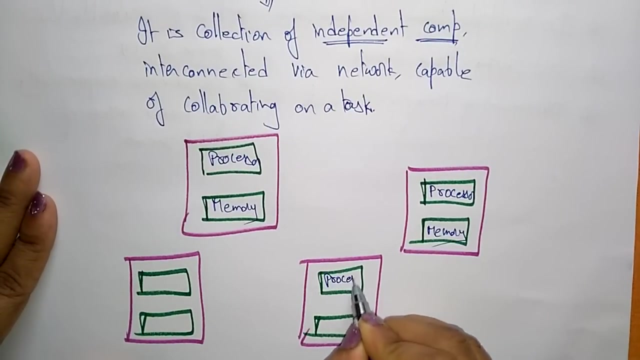 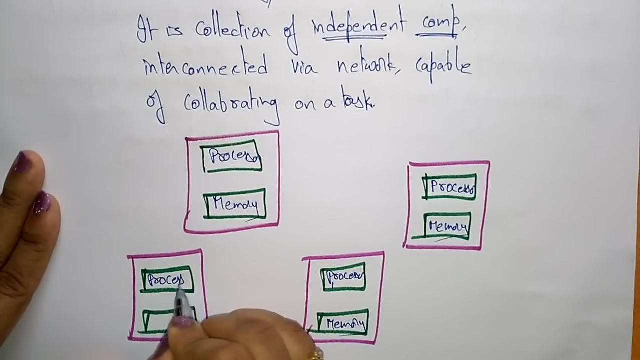 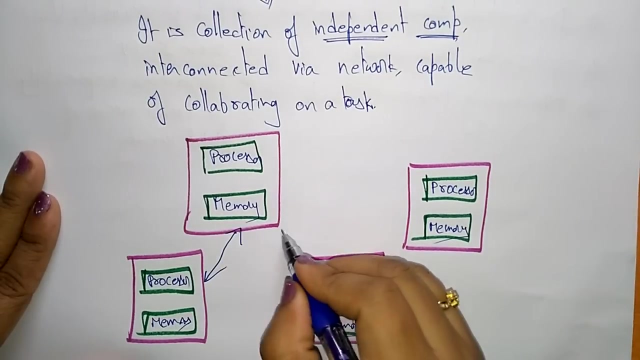 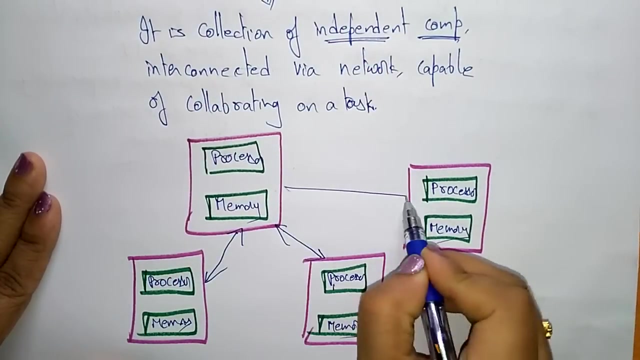 A different processor. Each system is having their own processor and memory. Each system is having own processor and memory, Processor memory. So these are all the independent computers, Processor memory, And this is also a processor and memory. So here one computer is connected to another computer. So this is an interconnected computers. So it is a collection of independent computers interconnected. So these are all interconnected via network and capable of collaborating on a task, And these are also capable of collaborating on a task. 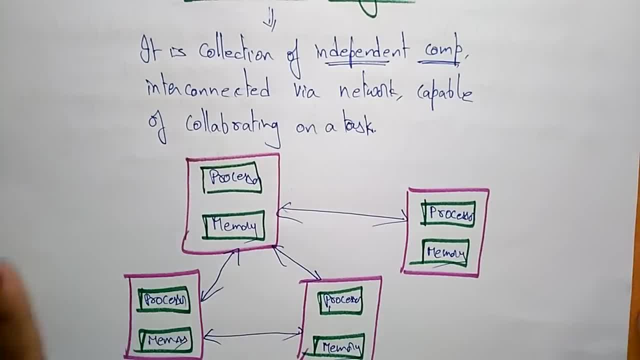 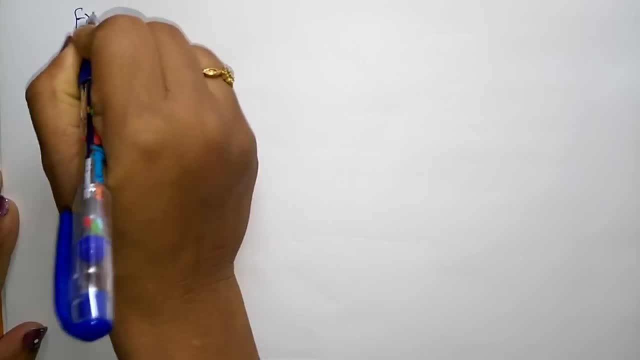 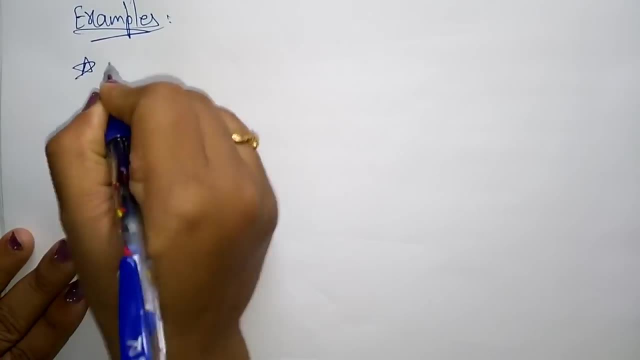 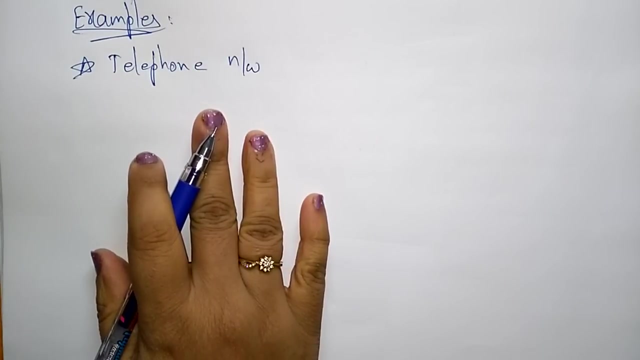 collaborating for a task. so this is about a definition of distributed system. now let us see what are the examples of distributed systems. examples, the examples of distributed system is telephone network. so in the telephone network also a connections, a telephone wiring that there is, it is following the 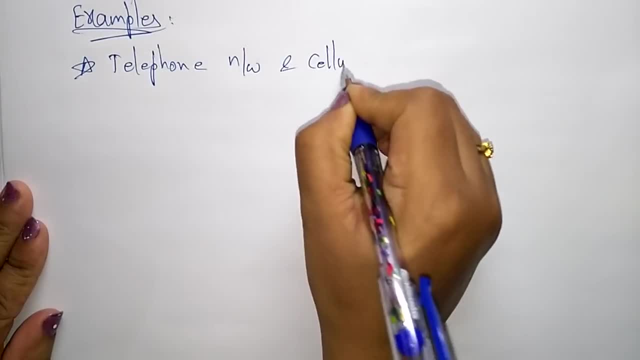 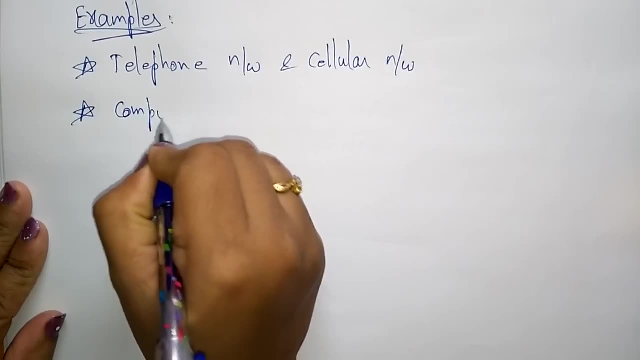 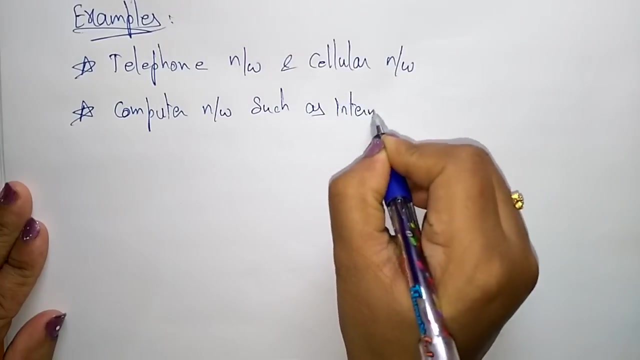 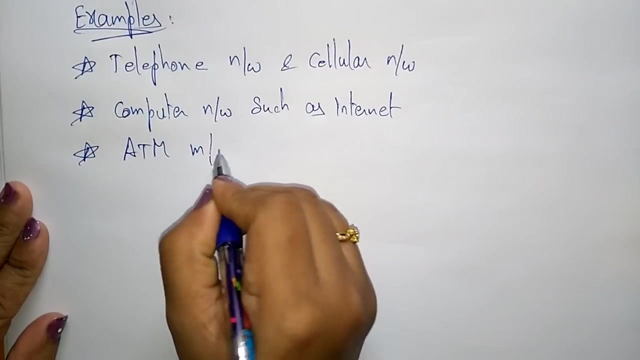 distributor technology and cellular networks, that is, a wireless and computer network such as internet network, such as internet, or you can take the ATM machines. so, whatever, we are using that ATM machines for withdrawing the money, so those ATM machines are also for is what type of distributed operating? 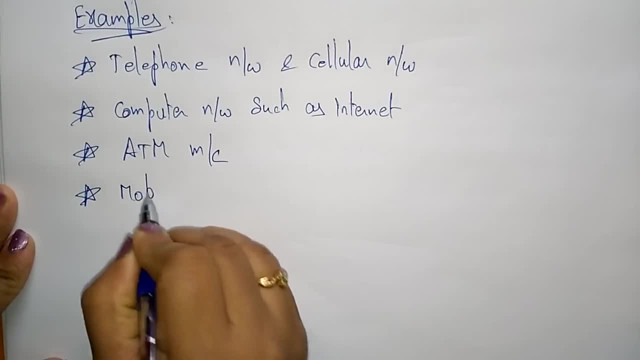 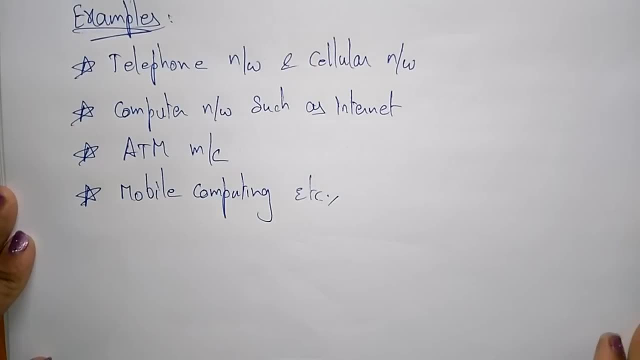 system is that. so that is the distribution technology, and then the distribution technology, and then the system and mobile computing, etc. so these system and mobile computing, etc. so these system and mobile computing, etc. so these are the different examples. the examples are the different examples. the examples are the different examples. the examples that, using the distributed operating, 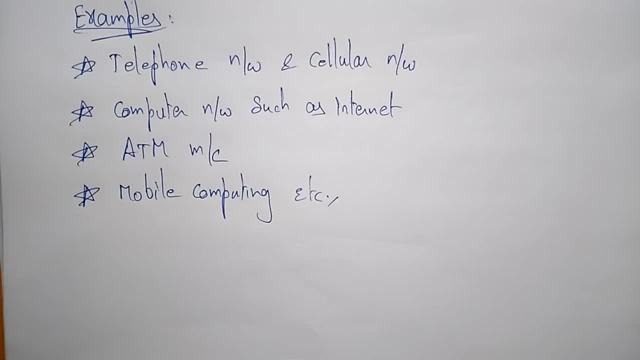 that using the distributed operating, that using the distributed operating systems. so let us see the one type of systems, so let us see the one type of systems, so let us see the one type of distributed operating system. so whatever distributed operating system, so whatever distributed operating system, so whatever we here, we have taken the examples, these. 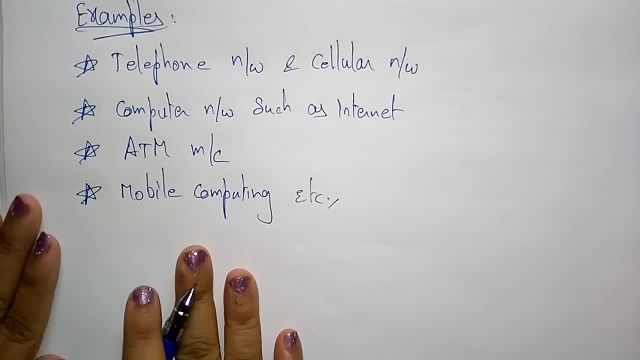 we here, we have taken the examples. these we here, we have taken the examples. these examples are following. examples are following. examples are following: a distributed operating system used as a. a distributed operating system used as a. a distributed operating system used as a client server systems. so let me these. 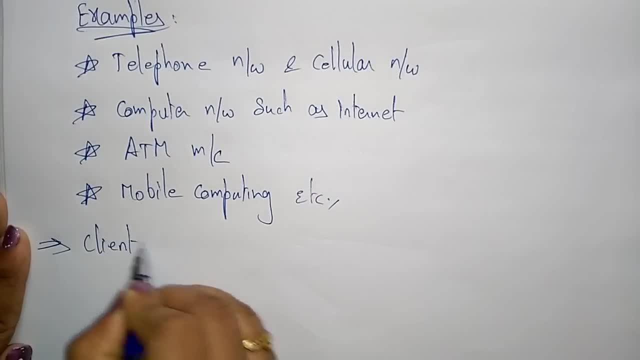 client server systems. so let me these client server systems, so let me these examples. follows the client server examples. follows the client server examples. follows the client server operating system means it is using the operating system, means it is using the operating system, means it is using the technology of client server operating. 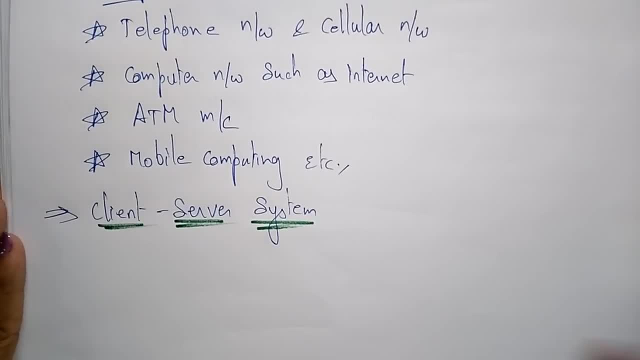 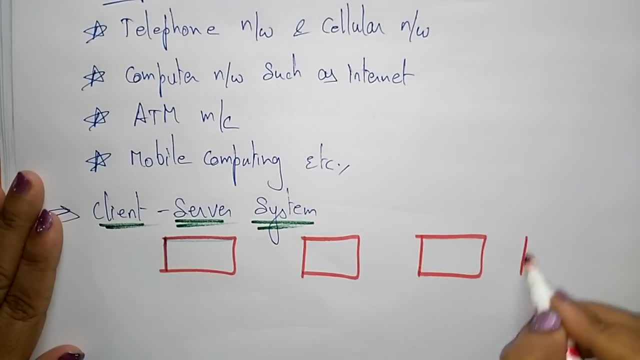 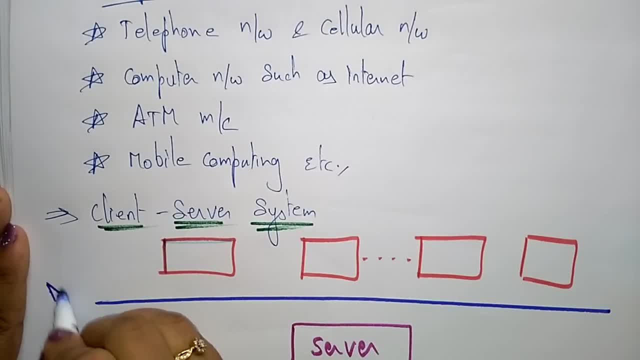 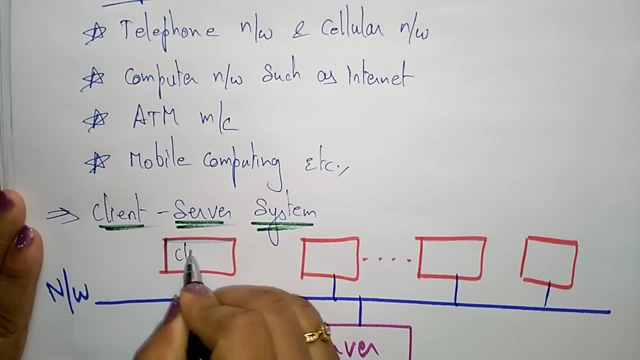 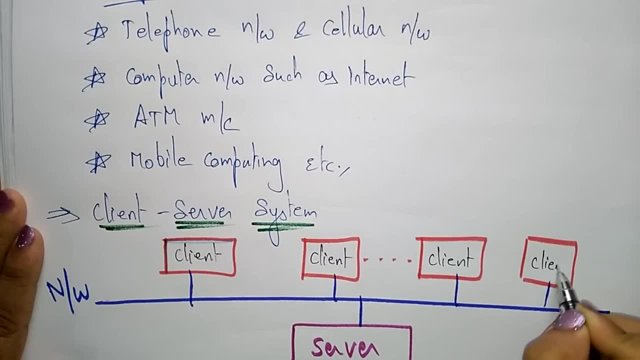 is a network, so this is all the clients. and the is a network, so this is all the clients and the server. so here client client line, so server. so here client client line, so server. so here client client line, so different clients, these are all clients. different clients, these are all clients. 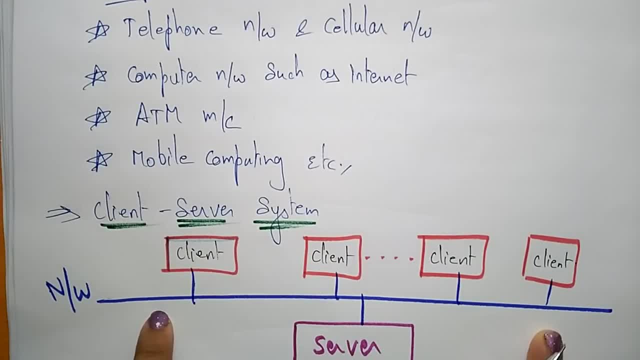 different clients. these are all clients are connected in using same network and are connected in using same network and are connected in using same network and that network is connected with server, so that network is connected with server, so that network is connected with server. so here this server is using by all the 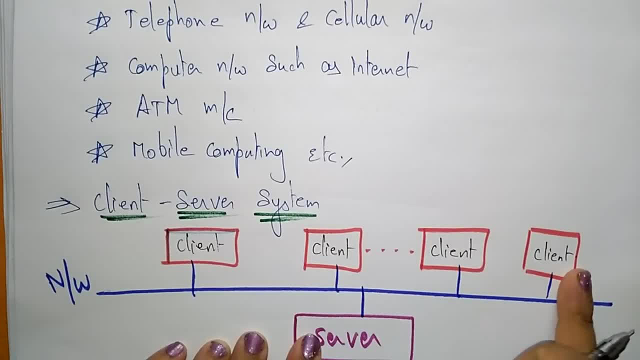 here this server is using by all the. here this server is using by all the clients. so a single server is using all clients. so a single server is using all clients. so a single server is using all the clients, the clients. so a single server is using all the clients. so this is a representation of client. 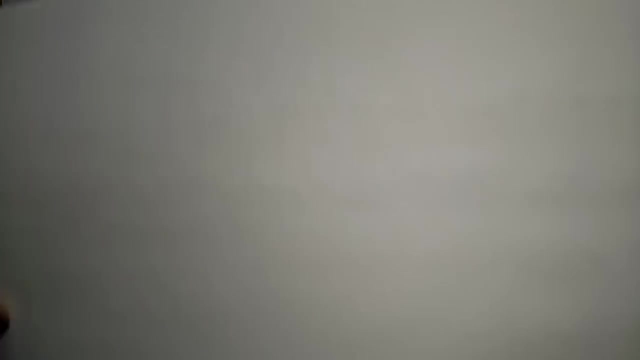 so this is a representation of client. so this is a representation of client server architecture. so here the server server architecture. so here the server server architecture. so here the server, broadly categorized as so. whatever the broadly categorized as so. whatever the broadly categorized as so, whatever the server we are taking, here this server. 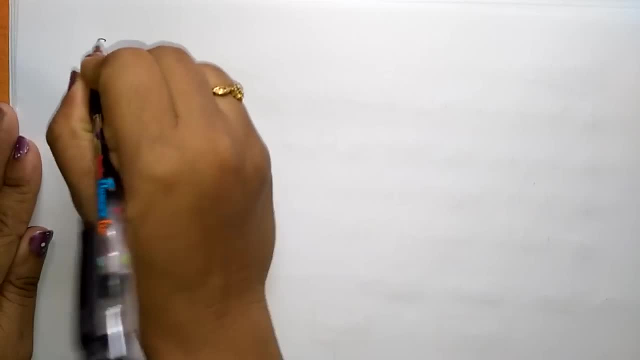 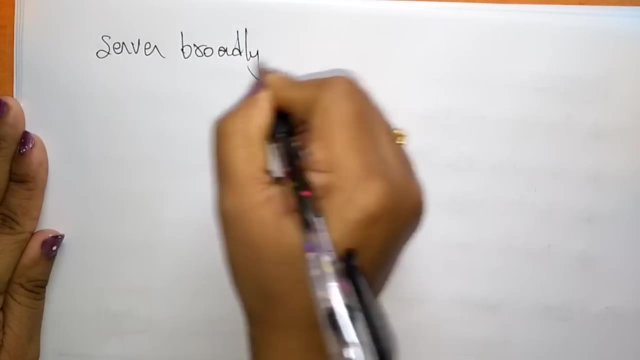 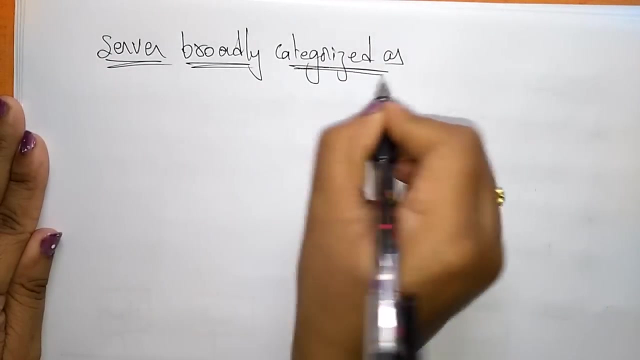 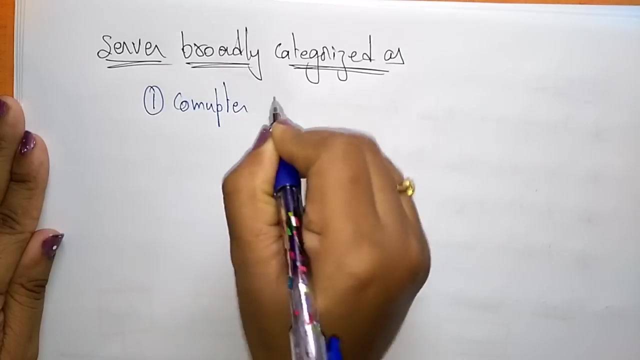 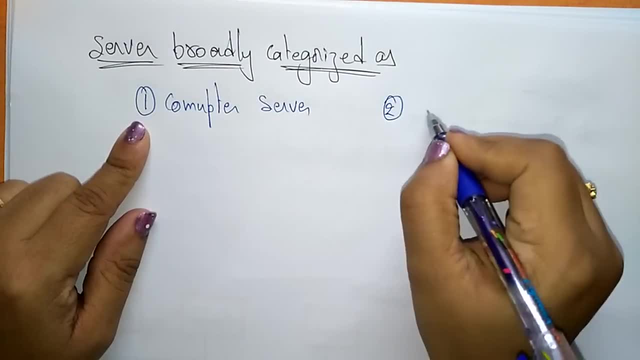 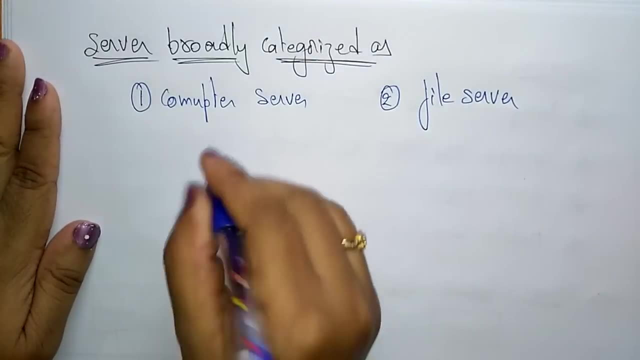 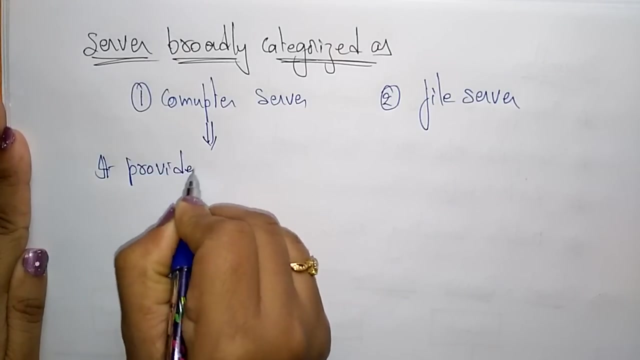 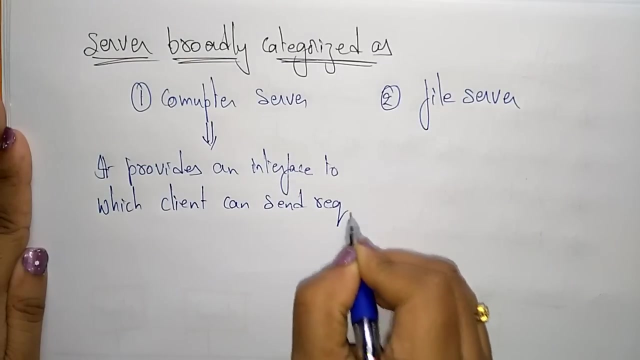 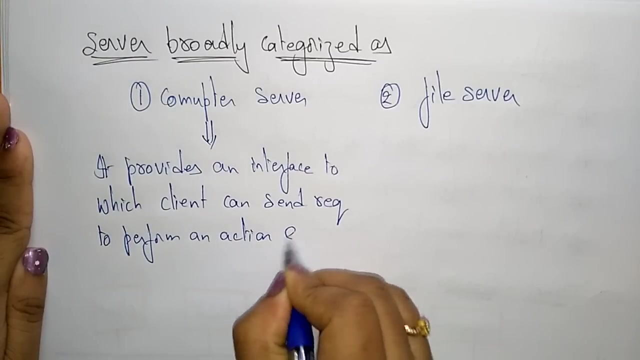 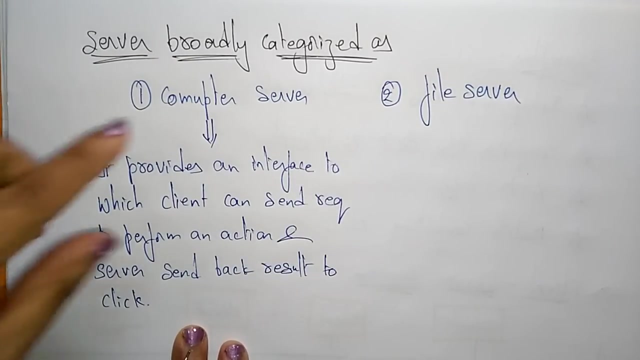 model. it may be a computer server or it must be a file server. computer server or file server, suppose if it computer server what it does. a computer server: it provides an interface to which client can send requests to perform an action and server send back result to client. so here a two-way communication is there in the computer. 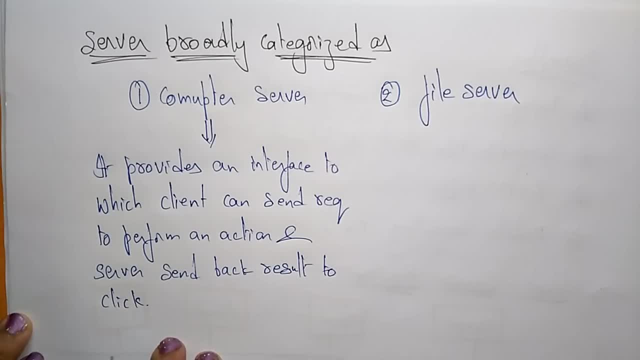 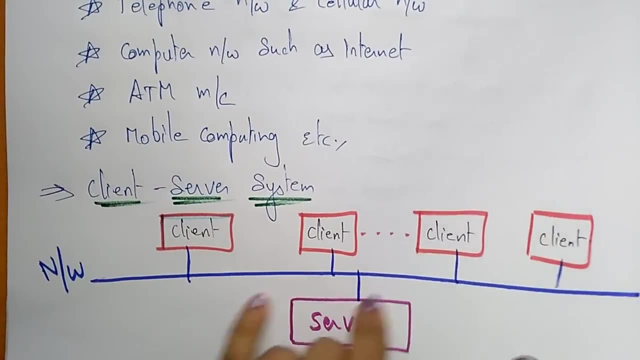 server. if you take a computer server, so first here the clients. whatever the clients are there, they are sending a request to the server. so whenever the server receives the info request from the clients, whatever the client that sends the request, the server again respond to that client request and send. 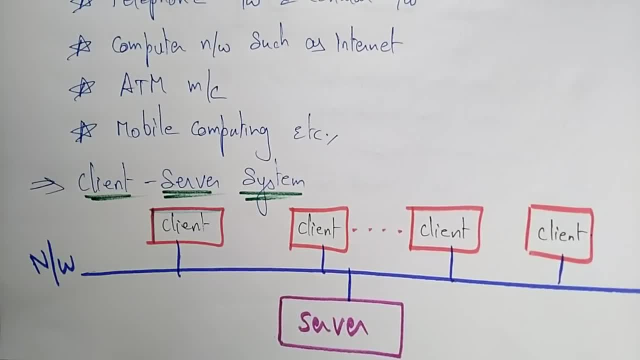 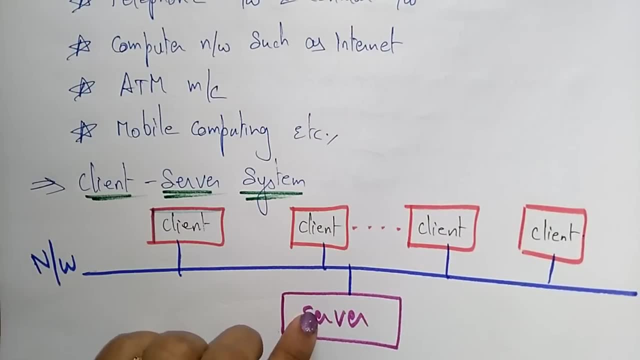 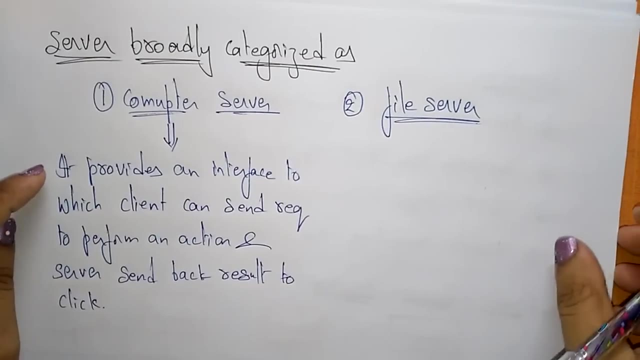 the data to whatever the client that is requesting you the message. so suppose this client is request the server to send some message, then the server will respond by sending the message that you call it as a computer server. so what about the file server? file server means is just a one. 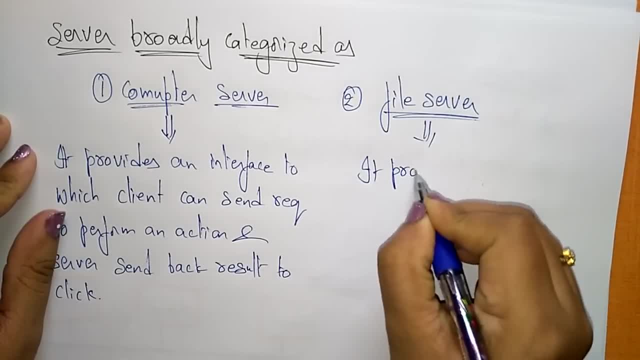 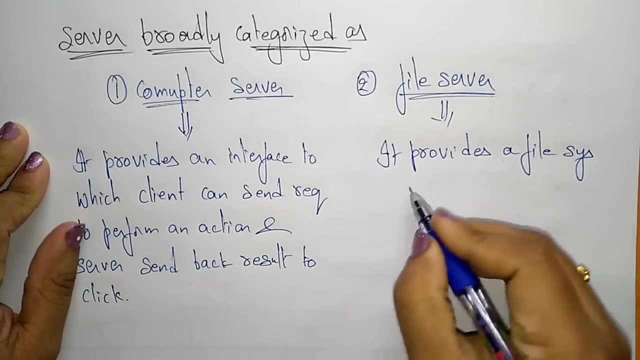 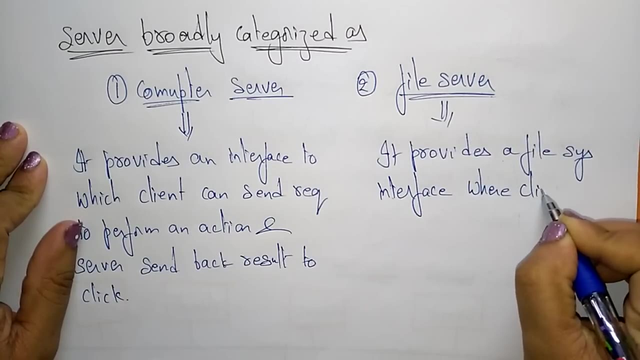 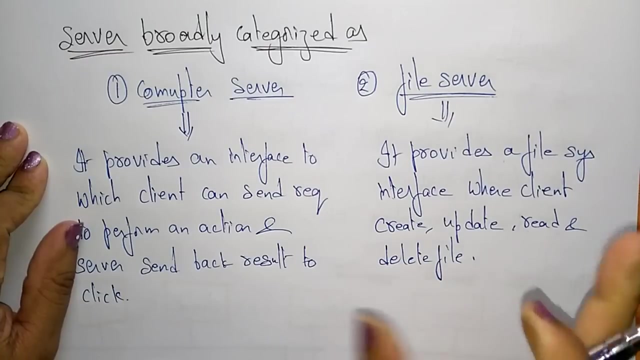 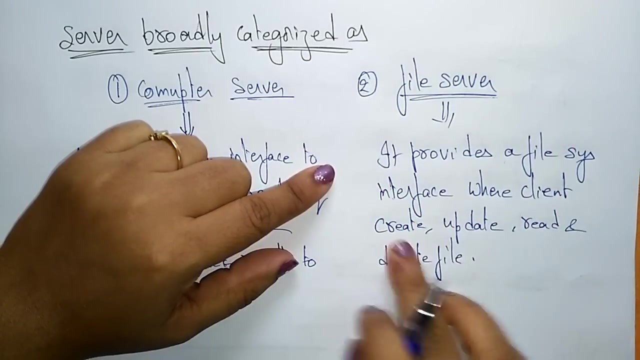 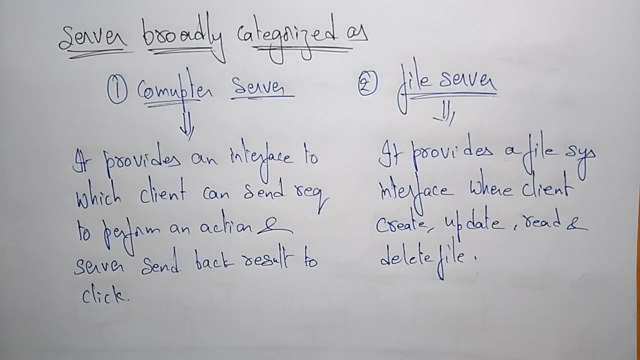 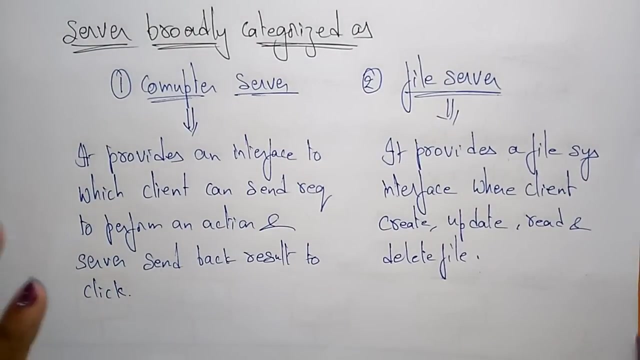 way it provides. it provides a file system interface where it provides a fight system interface where client can create, update, read and delete files in the file server, for example, the future client, therefore someone is received is regard that as a comment, categorized as computer server as well as it may be a file server. so here the the main. 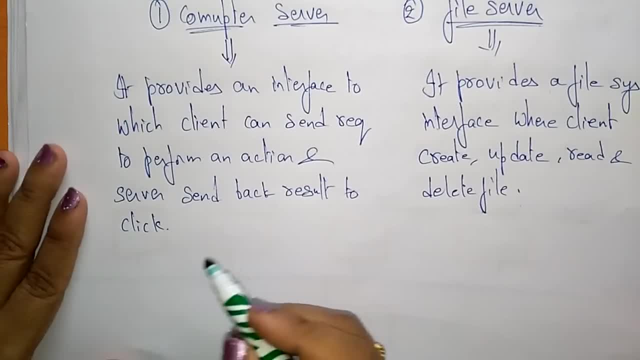 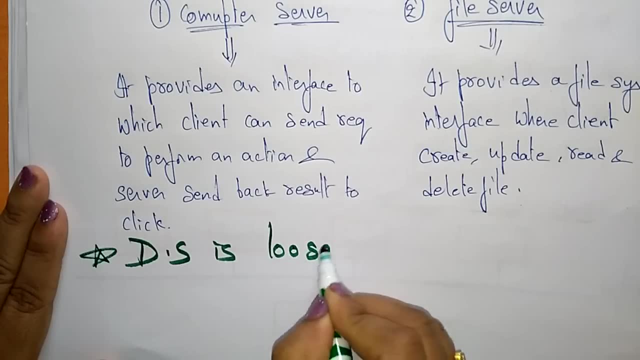 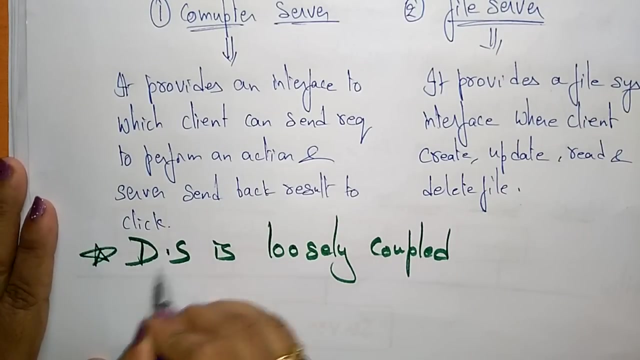 this distributed system is a distributed system is loosely coupled. we call it as a loosely coupled. so why we call it as a loosely coupled? distributed system is loosely coupled because here there is no shared memory. a distributed system is a loosely coupled because there is no shared memory, because each system is independent to other system. each system is having their own. 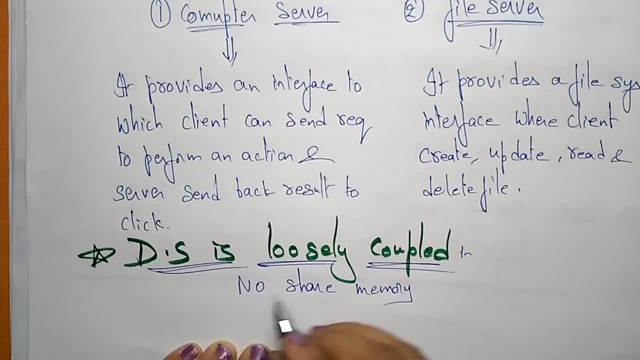 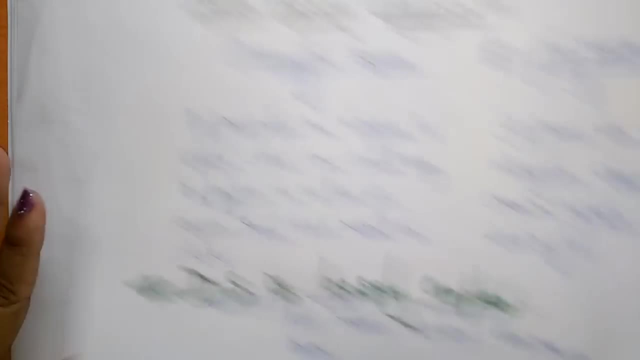 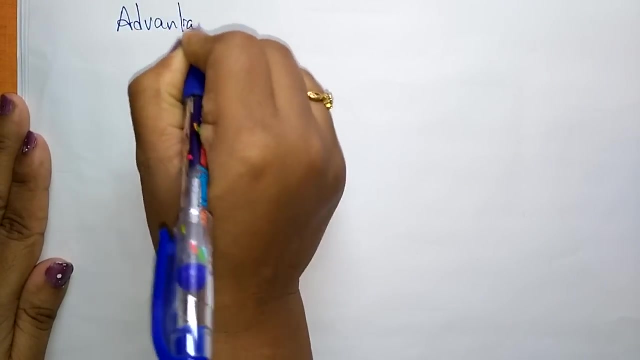 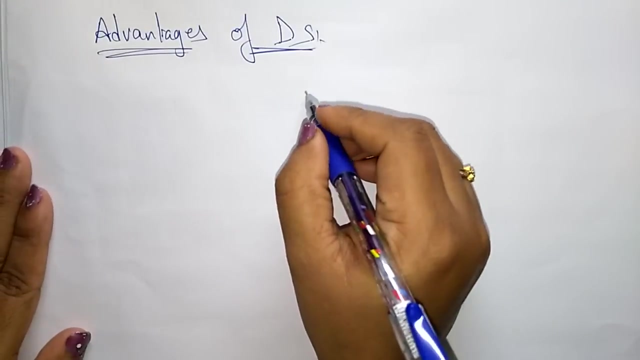 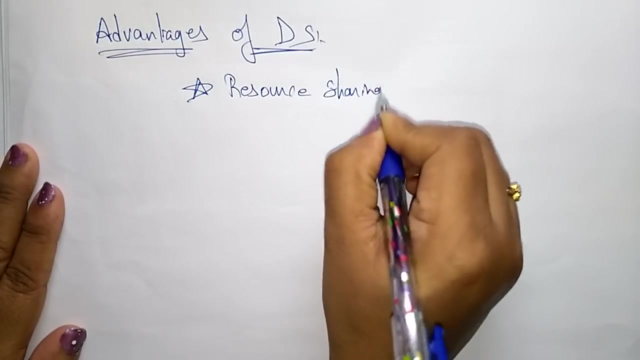 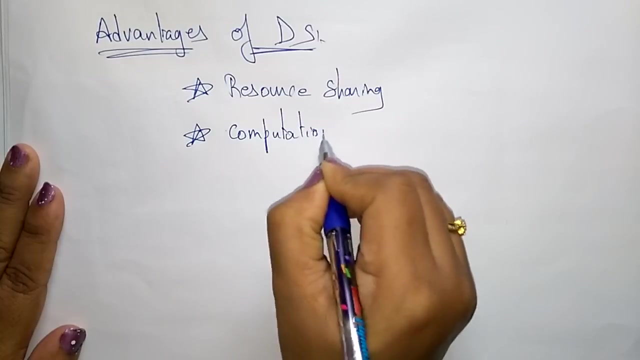 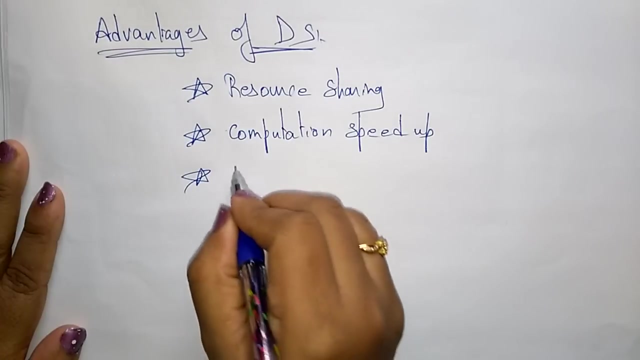 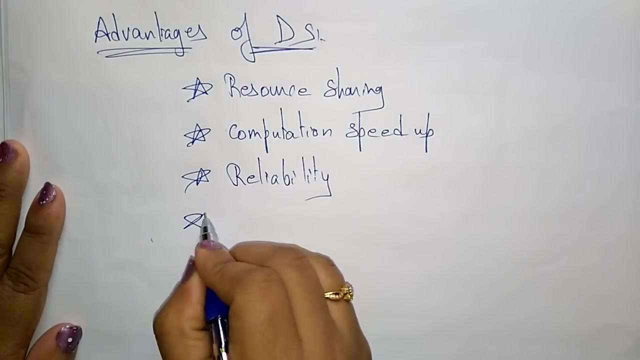 processor and the own memory. so no shared memory. various communication lines will be there, so that's why distributed system is a loosely coupled. then what are the advantages of this distributed system? advantages of distributed system? the advantages are resource sharing. resource sharing, computation. speed up computation. speed up. next, reliability: reliability and communication. 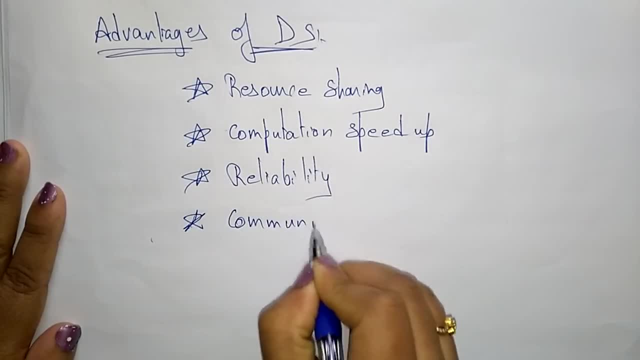 communication. so communication, just a via example for communication is email, so this is about the advantages of distributed systems. thank you,